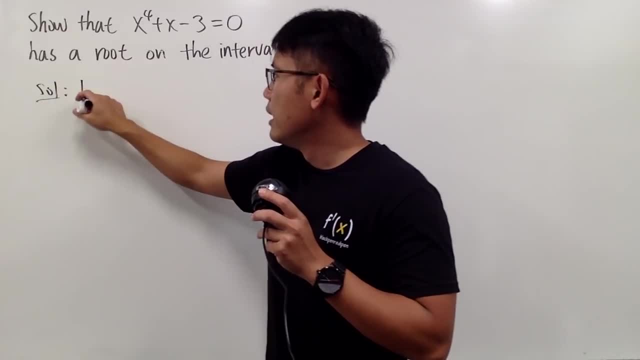 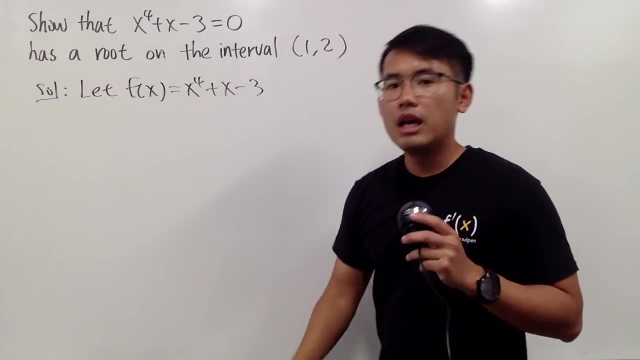 So I'm going to just go ahead. Here's my solution, Starting by that the function be that x to the force power plus x minus 3.. And if this equation wasn't equal to 0,, then of course we can just: 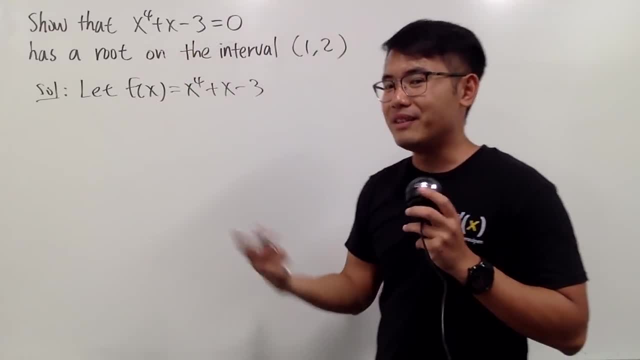 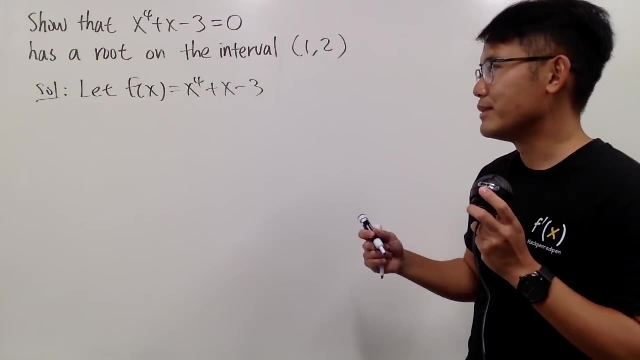 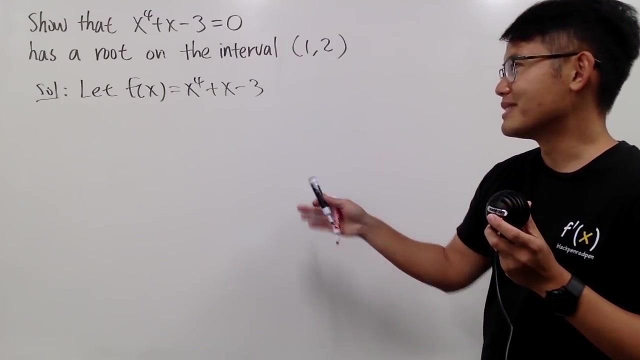 move the things on the right hand side to the left and then define the left hand side to be the function, right? So I'm going to define this to be the function And I will have to tell you guys that, you see, this is just a polynomial right And the best thing that you can remember is that. 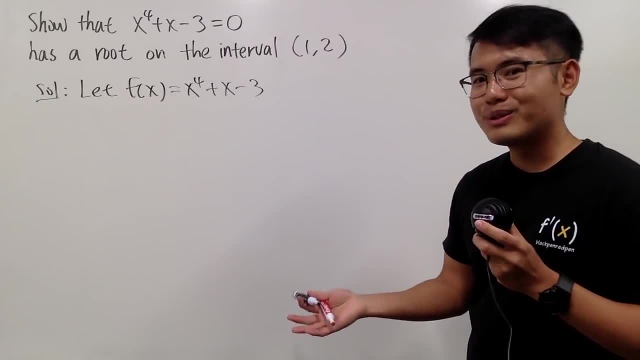 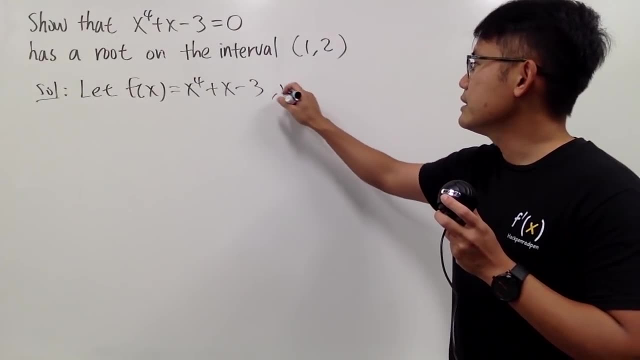 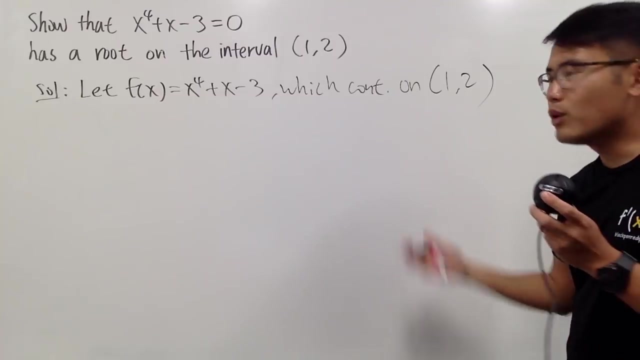 there's no fraction, there's no denominator, there's no square root, there's nothing that will bother you. So you're just going to say that this is the function, which is continuous on this interval 1, 2.. And, of course, for the endpoint. sometimes people put a square bracket to include endpoints. 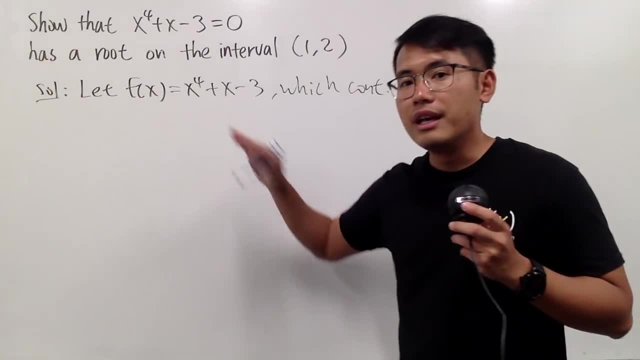 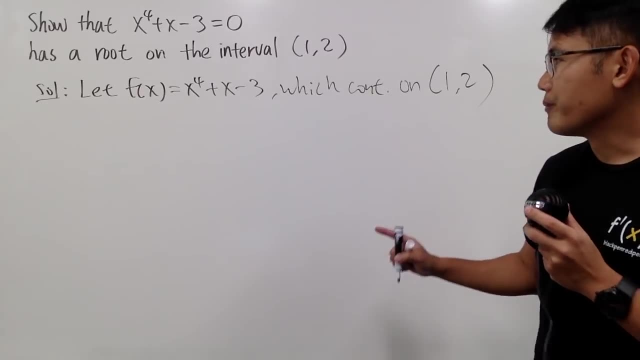 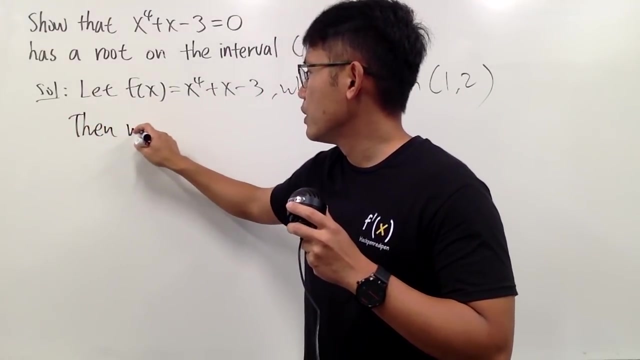 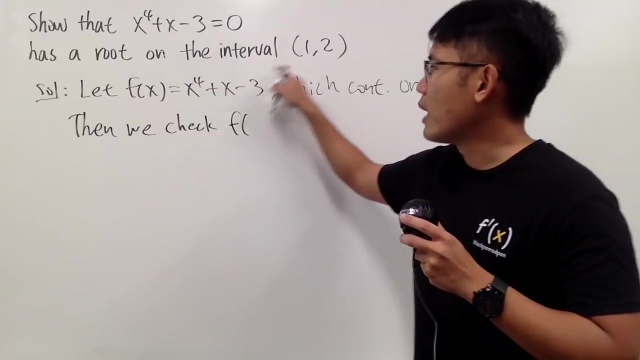 In this case it doesn't really matter, because this right here is in fact continuous everywhere. There's no fraction, no square root right, Just a polynomial. So here we have this continuous function Right here. Then we check the endpoints of this interval. So I'm just going to plug in 1 into this function first. 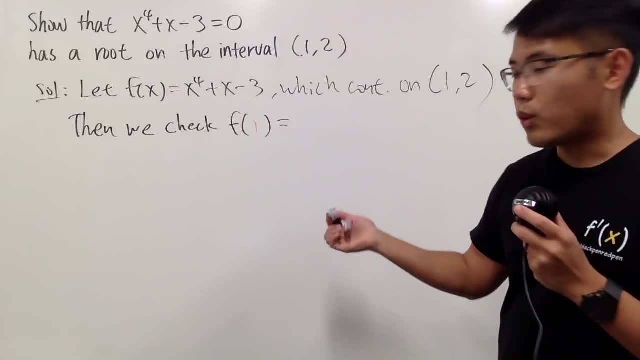 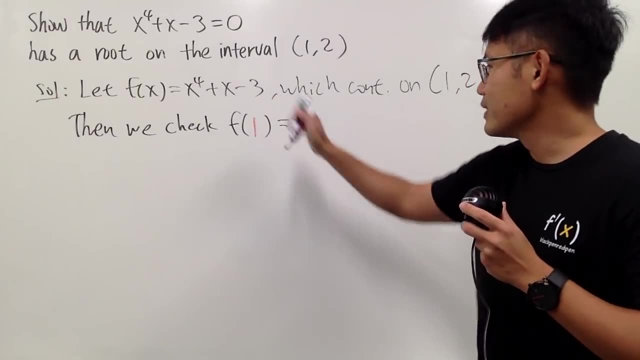 We are going to check f of 1. And we have to see what does this equal to? And let's just go ahead and do the math right, All right, So plugging 1.. So we have 1 to the fourth power plus 1, and then 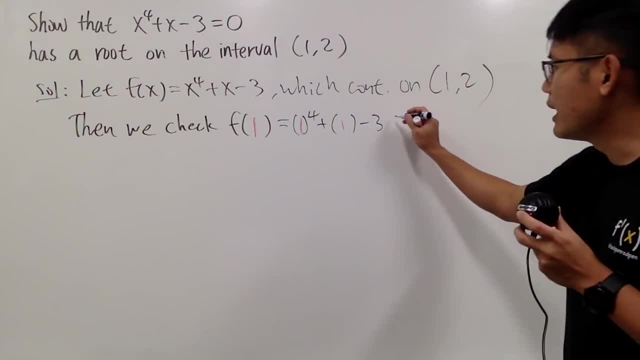 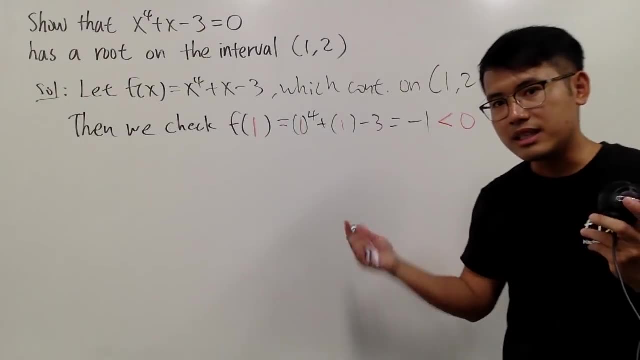 minus 3.. This is just 1.. Plus 1 and then minus 3.. So you get negative 1. And you have to indicate that this right here is less than 0, right, It's a negative number. And we also check f of 2. And we do the same thing. 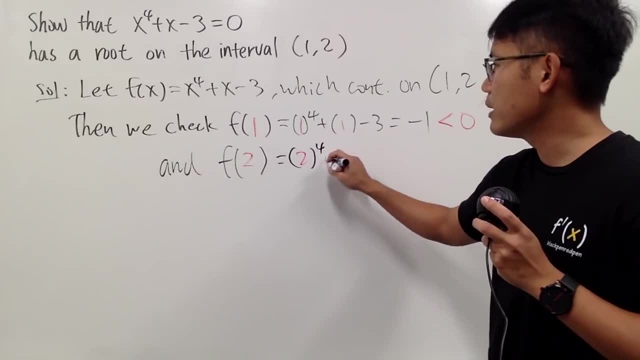 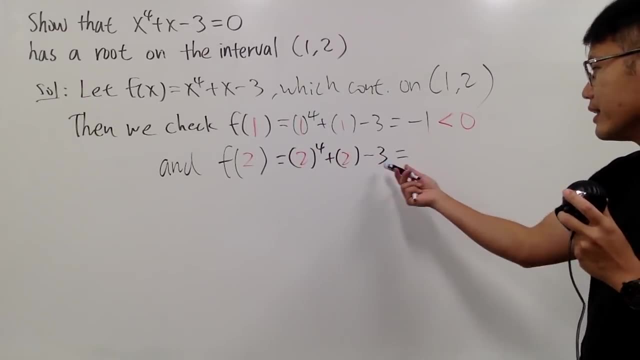 You plug in 2 into x, So you have 2 to the fourth power, and then plus 2.. And then minus 3.. This is 16 plus 2 is 18.. And then minus 3 is 15.. And, most importantly, 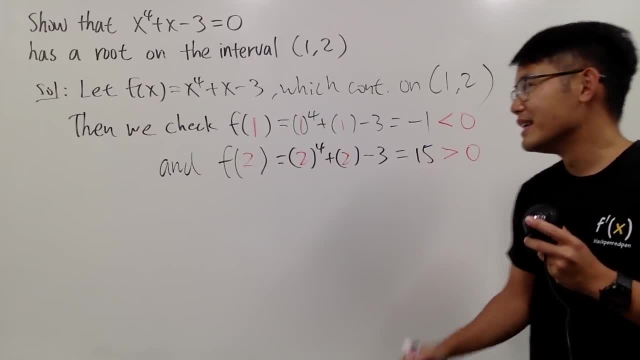 15 is negative 1. So you get negative 1. And you have to indicate that this right here is less than 0. And then minus 3 is positive, right? So here's the deal. You have a continuous function. Let me.